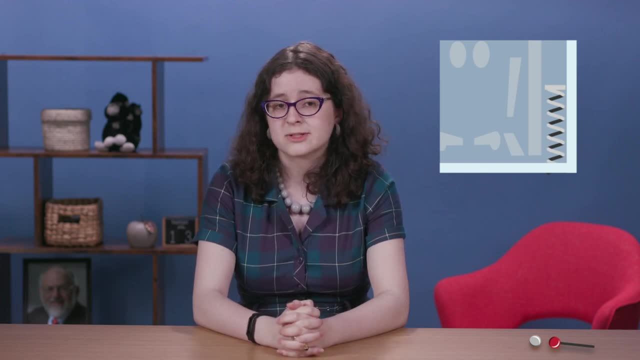 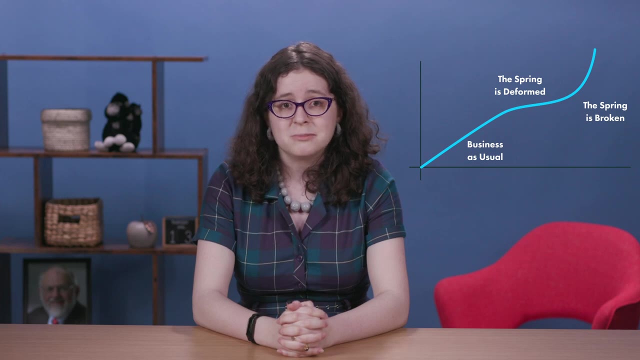 changing the relationship between how hard the plunger is pulled and the force on the pinball. While the relationship is linear within the elastic limit of the spring, the relationship between how hard the plunger is pulled and the force on the pinball isn't actually. 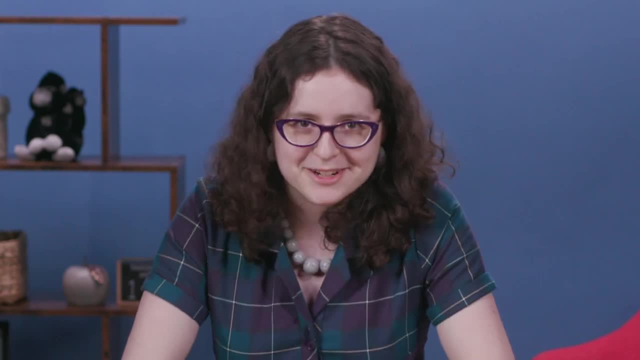 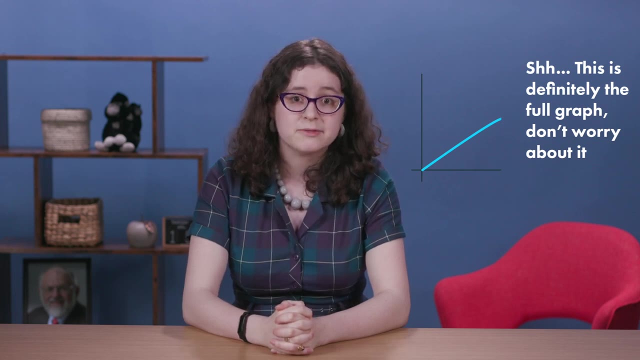 linear. However, we can model the spring of a regular pinball machine as an LTI, as long as we model it within the elastic limit of the spring. We can make sure our spring, with set elastic limit, can handle the range of human strength And hope our pinball machine doesn't. 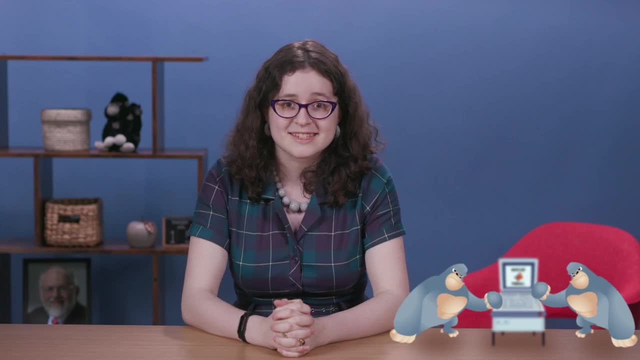 get too popular among silverback gorillas. An ultimatum: They target as many humans as possible. That's the philosophy of the formula: Come on贴 그거. come on, you play for a very long time, I don't care about anything. 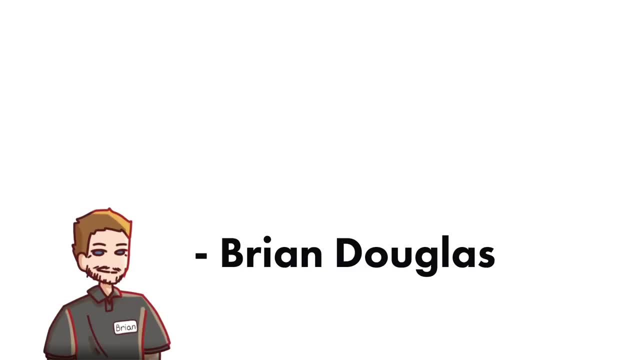 And to that end, we've already been informed you f Jayden Bell told him to keep Dante de Conti at a Alma's reception chart over the n рок MAX show. Why design controllers with LTI systems? Well, to quote Brian Douglas, quoting Richard Feynman, 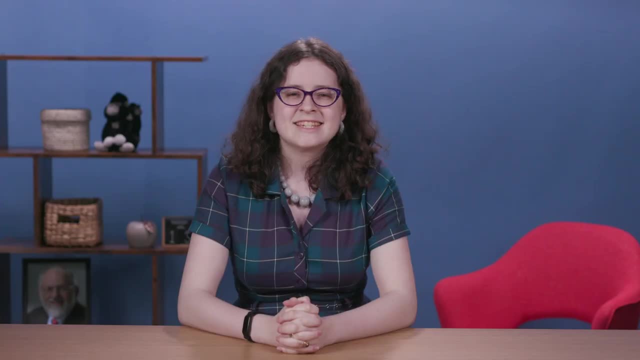 linear systems are important because we can solve them. This isn't to say that we can't use nonlinear systems for control design. It's just that linear systems are significantly easier to model and work with. We can get to a linear or linear time invariant representation. 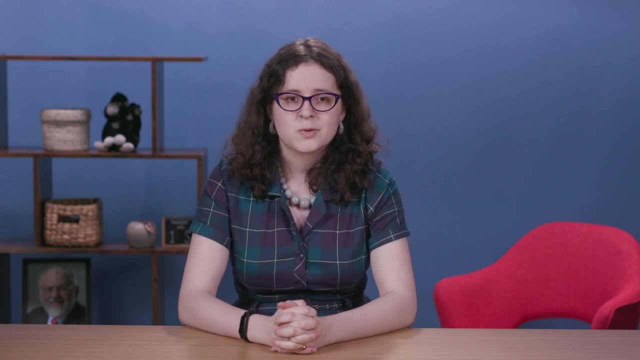 of a nonlinear system by using transfer functions. Transfer functions are derived using differential equations and the Laplace transform. If you're anything like me, the phrase differential equation sets off your fight or flight response. Learning DiffEQ was hard enough the first time around. 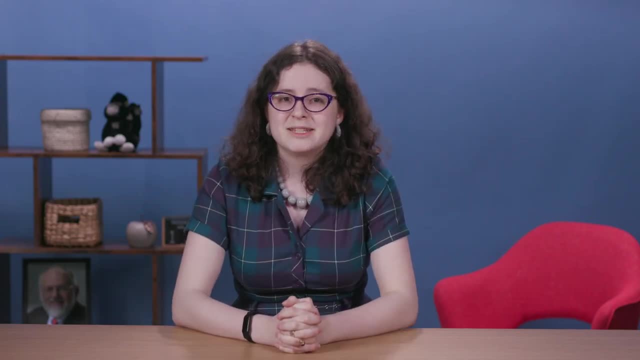 and I'm not doing it again. Fortunately, with MATLAB and Simulink you don't have to derive the transfer functions yourself. The computer does it for you. Let's take a look at using Simulink in a real world example. 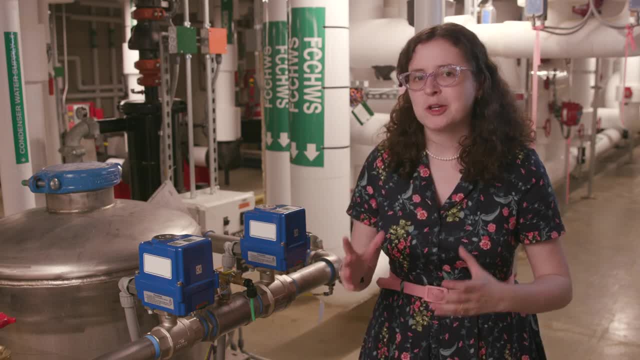 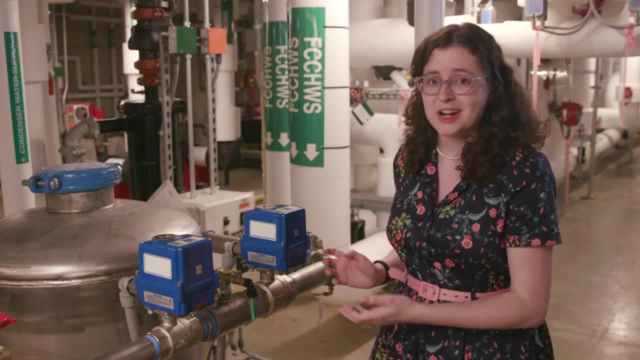 In this example, we have a water tank and we want to maintain a particular water level in the tank. Essentially, our system is made up of a water tank and two valves- one that lets water in and one that lets water out- and a sensor inside that. 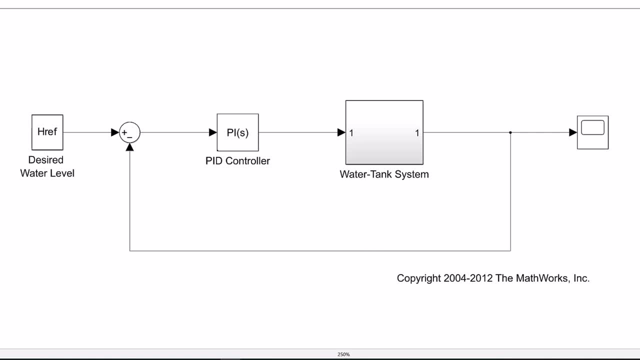 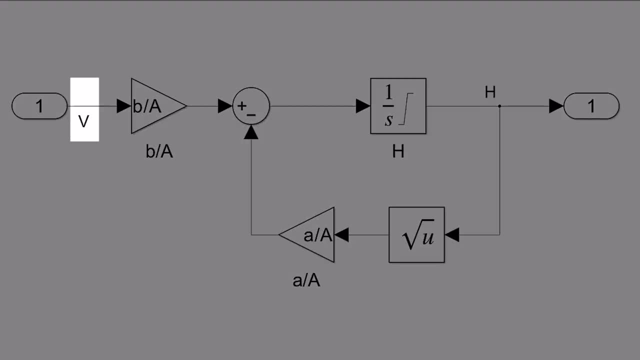 tells us our current water level. Here's what the overall model looks like in Simulink. If we double click the water tank, we can see the system equations for the tank. The input to the system is the voltage to the valves, which determines by how much the valve should. 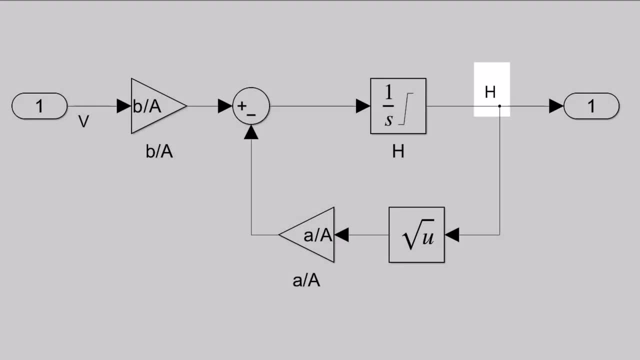 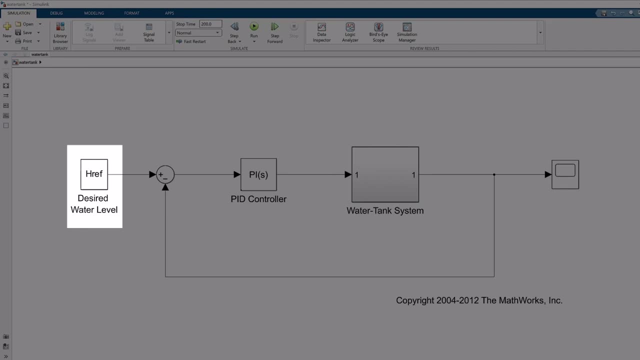 be opened or closed And the output is the measured height. If we go back to the top-level model, we can see that the water height is fed back into the system so we can compare it to our desired water height. Based on that difference, we feed. 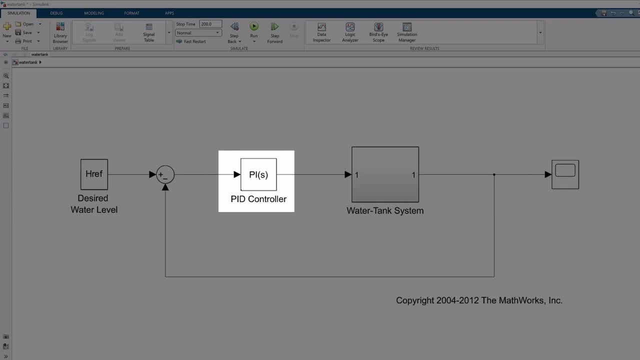 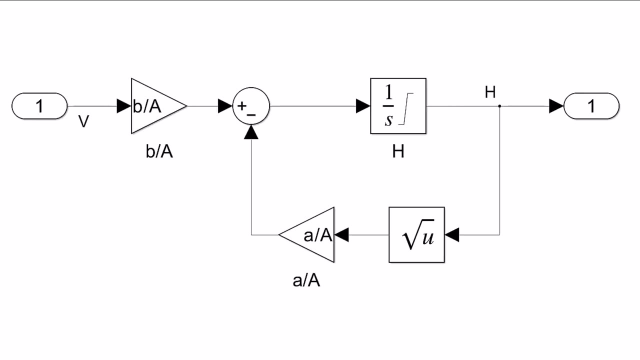 the value into the controller to generate a particular voltage for our valves in the water tank system. Now, this is a simple nonlinear system. You can see here that there's a square root in the system of the tank. Having a linear model of that it's very tasty. 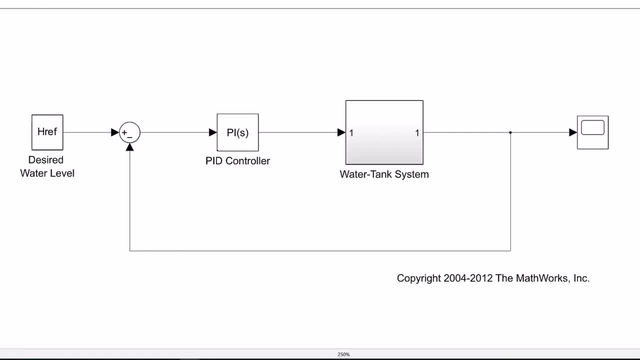 this system makes it easier to tune a controller such as a PI controller. The first step to linearize this system is to specify linear analysis points, in our case with the input of the voltage and the output of height. We left-click the signal here and set analysis points and then go to the app section of the tool. 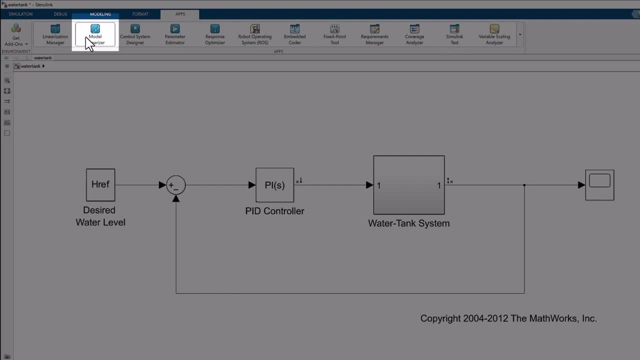 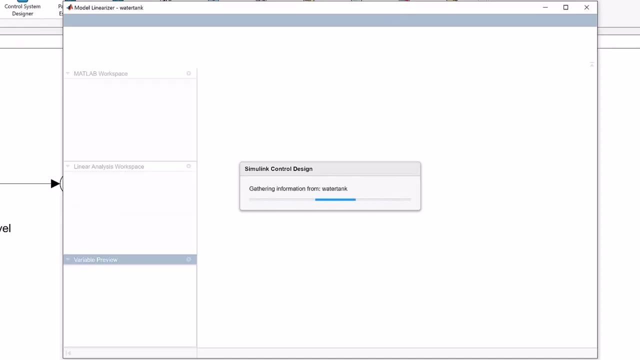 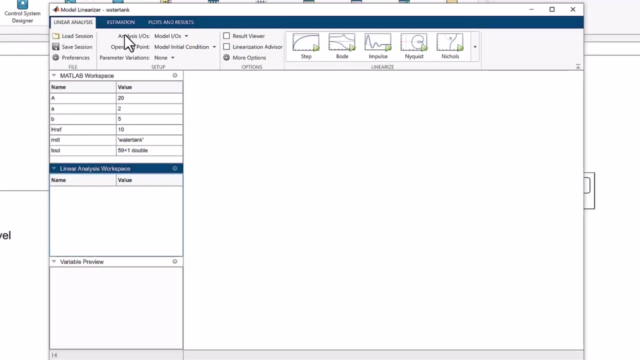 strip and select the model linearizer. As one might suspect, this app helps us get linear representations of our nonlinear systems to aid in control design. In the model linearizer we need to select the operating points. In this case, we're okay. 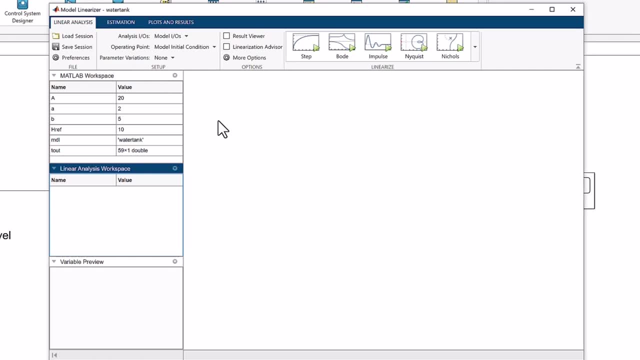 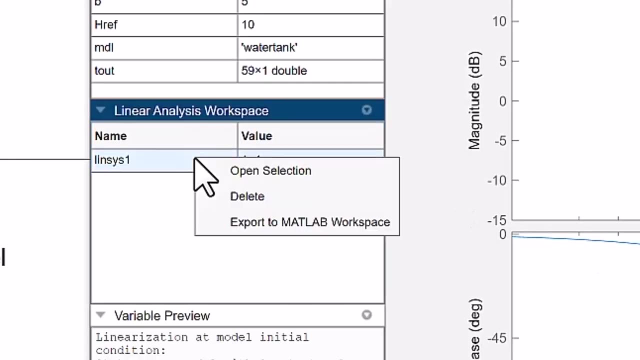 with linearizing the system with the initial water level of the tank, and so we select the model initial conditions from the drop-down. When we linearize the system at this operating point, we get the linear representation as a state space model. However, we can convert this state. 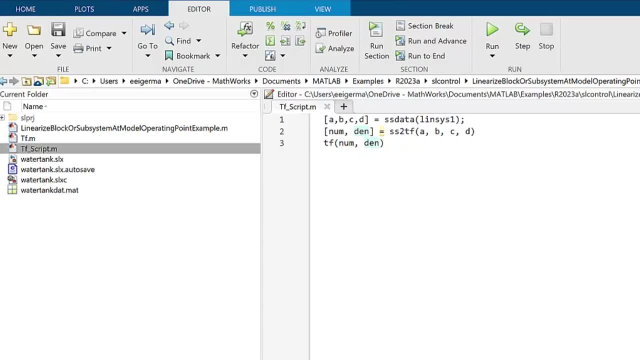 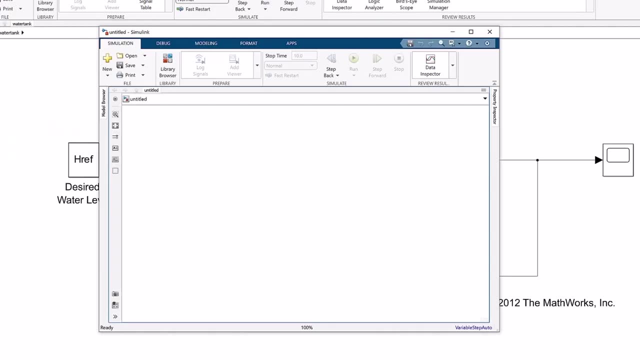 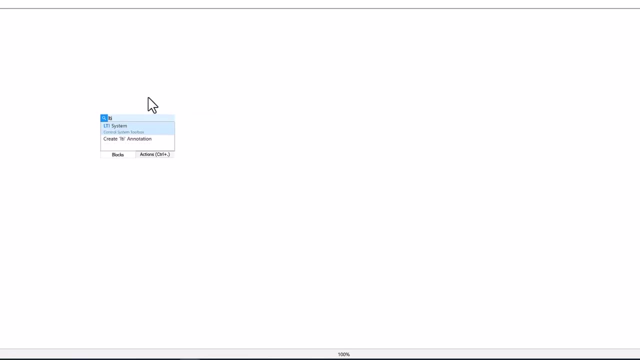 space model into a transfer function by exporting it into MATLAB and using the SS2TF function. With the transfer function we can create a new model where the water tank system is represented with an LTI. We place an LTI block in our model and call the LTI model from our MATLAB workspace After the system has. 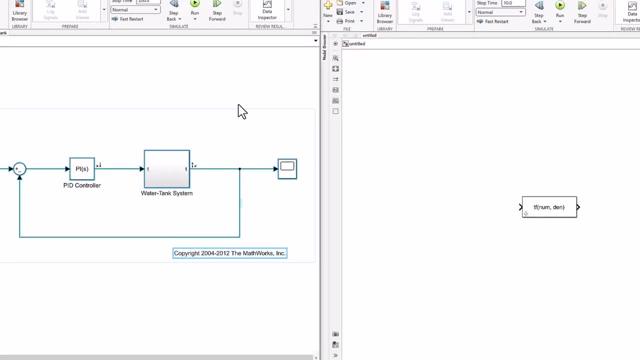 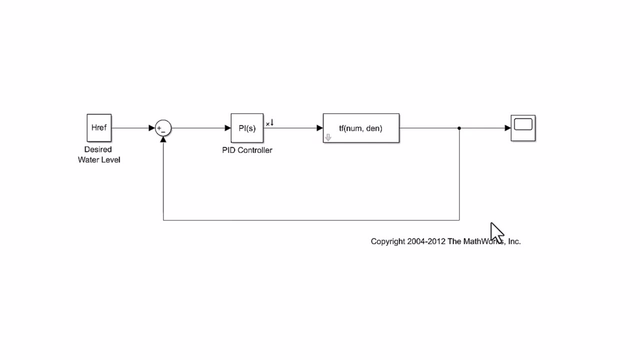 been replaced. we can bring over components from the previous model and tune our controllers. Now we have a linear representation of our model that we can use to do control design and analysis in MATLAB and Simulink, But you don't even need to go to that. 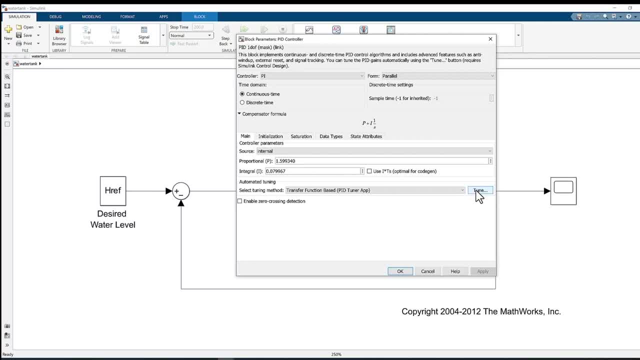 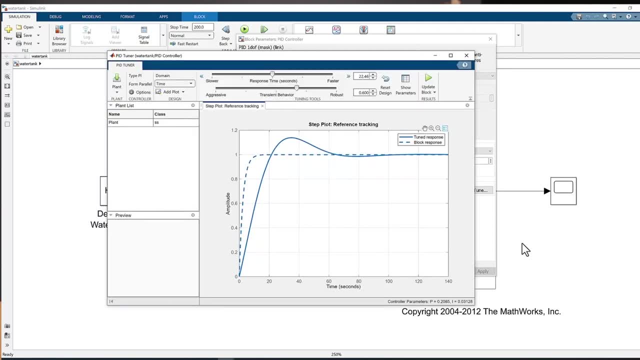 much trouble to tune a PID controller. The PID tuner app does the linearization and tuning for you automatically. But now that we've seen the workflow in a simple system, let's take a look at the same process in a more complex system, In. 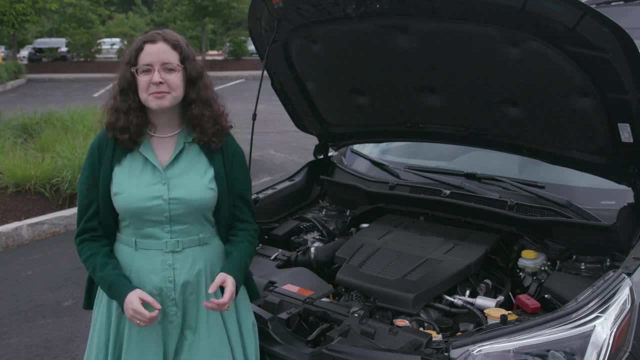 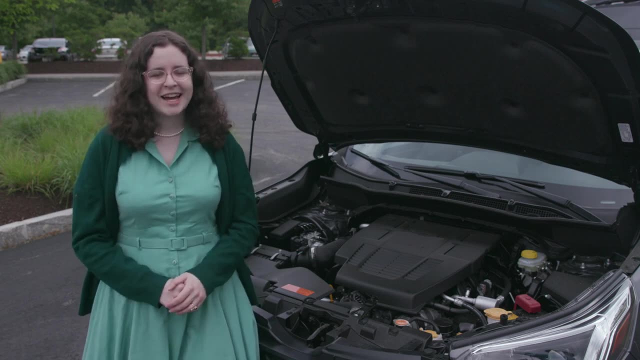 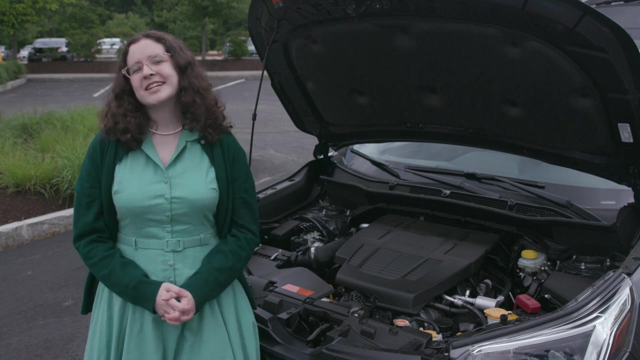 an engine control system. the goal is to maintain a particular number of engine revolutions per minute in relation to how hard the driver is pushing down on the pedal. As one can imagine, an engine control system has significantly more going on than just a tank with two valves. Let's take a look at the system. 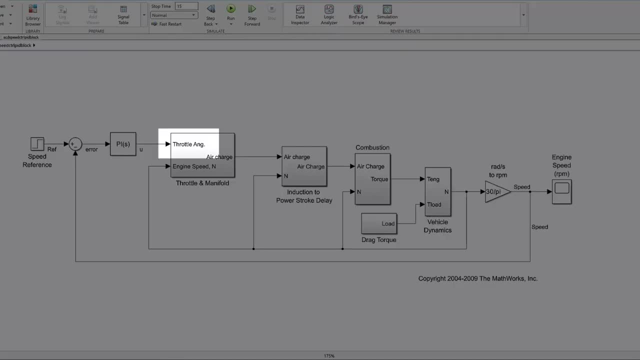 in Simulink, Our input is the throttle angle and our output is the engine speed. We have four separate systems: Throttle and manifold, induction to power, stroke, delay, combustion, drag, torque and vehicle dynamics. We're trying to design a controller that gives the desired 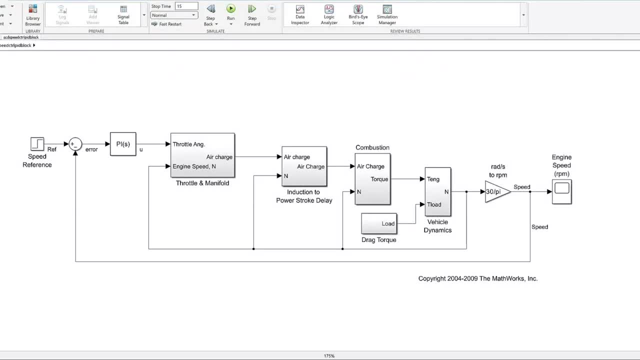 engine speed for a particular throttle input. To achieve this aim, we need to design a PI controller for this complex nonlinear system. However, unlike, say, water valves, the system dynamics of our system varies at different engine speeds. Tuning a single PI controller would not provide a good controller performance. 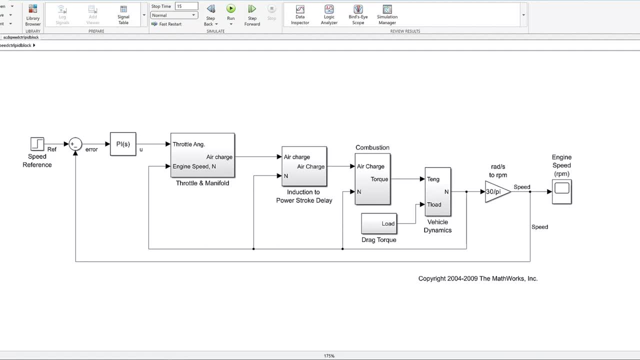 across the entire system. So we need a gain-scheduled PI controller that can adapt the gains depending on the engine speed. In order to do that, we need to generate LTI representations at different operating points of the engine and use it to tune PI controllers. Let's take a look. 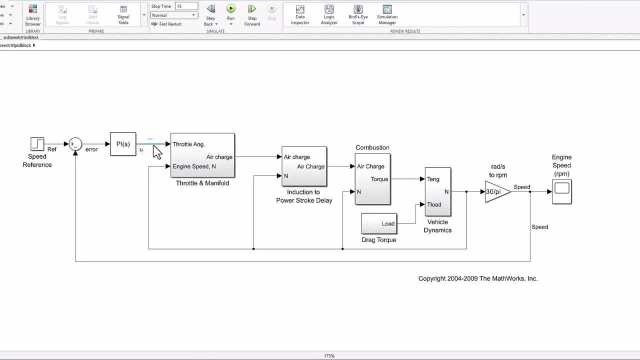 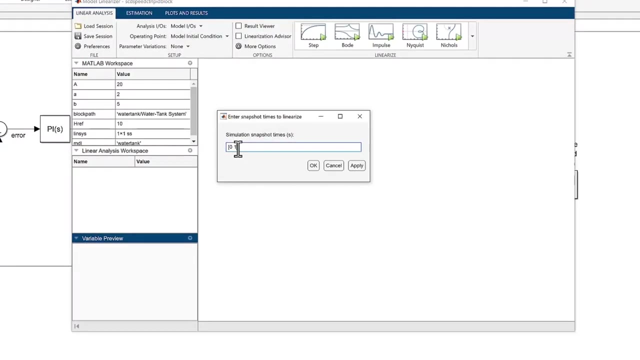 at how to do just that. The premise is the same. We put the linearization points at the inputs and outputs of the model. Before we can run the model linearizer, we need to select an operating point. In this case, we choose the operating point of 6 seconds. 6 seconds is when the engine is in a steady 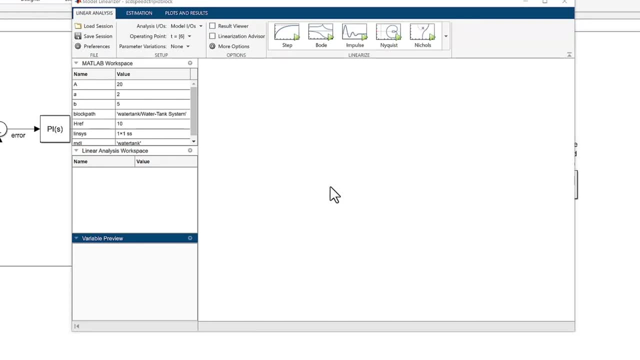 state. Now that we have the operating point and linearization points, we can run the model linearizer. You probably won't be surprised if you see that the engine is in a steady state. when the engine is in a steady state at 6 seconds, For instance, the engine is in a steady state. 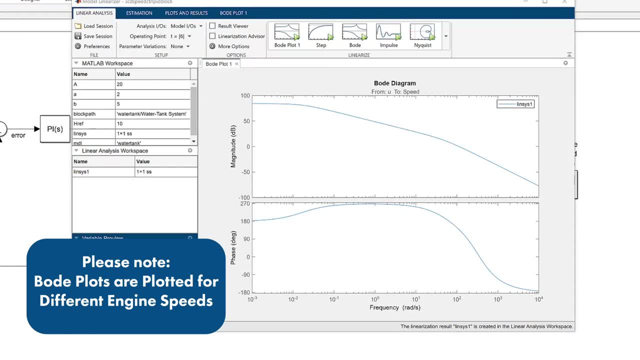 when it is in a steady state at 0.8 seconds. But a model for just 6 seconds isn't enough. We need a linear representation at two throttle inputs, Maybe one at 8 degrees and the other one at 8 and one at 2.. 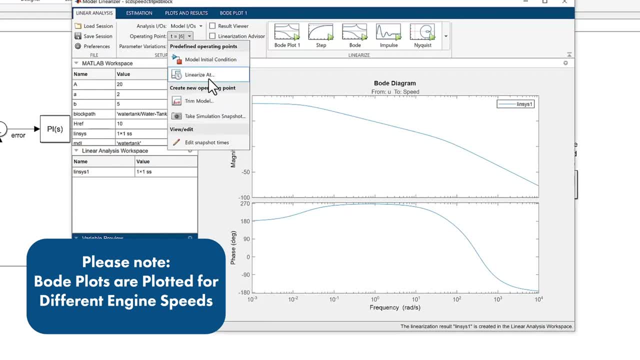 Then we need to evaluate the model, to select the model that we want to use. We need to one at 20 degrees. At 8 degrees the engine settles at 6 seconds and at 20, at 14 seconds We are going to shift the operating points. 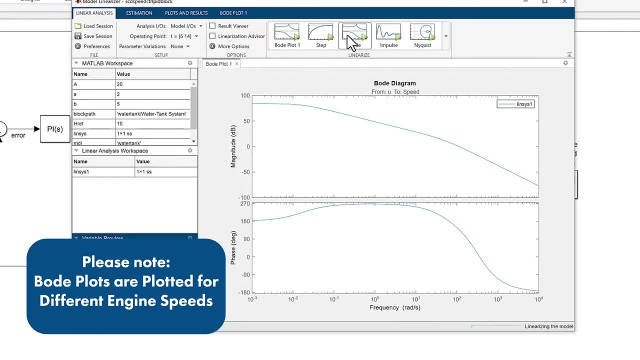 to 6 and 14 seconds. We get two models by running the linearizer and we can use the models between these points to get a linear representation of the system. But this is all well and good if you happen to have a Simulink model of your system. 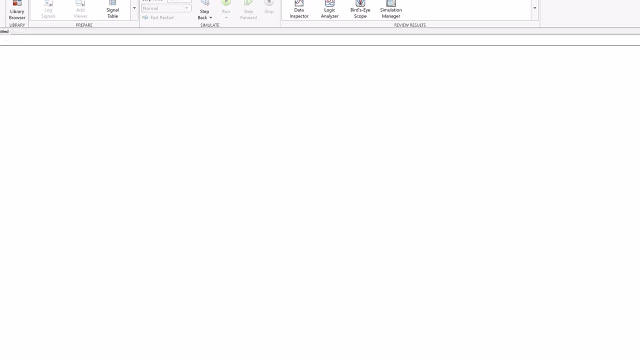 What if you don't have time to construct a model, or bought an engine from a manufacturer and don't have knowledge of the inner workings of the engine system? We can put some gas in the engine, fire it up, press the throttle and record the engine speed. 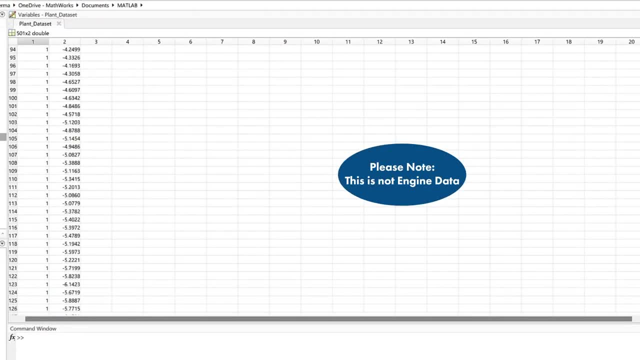 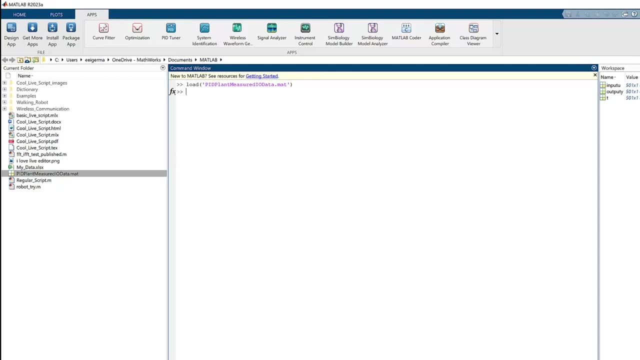 at different throttle positions, giving us a set of inputs and outputs to work with. Once we've imported the data into MATLAB, we can do system identification to fit transfer functions to the data. We can let the PID tuner automatically fit a transfer function or we can do it ourselves. 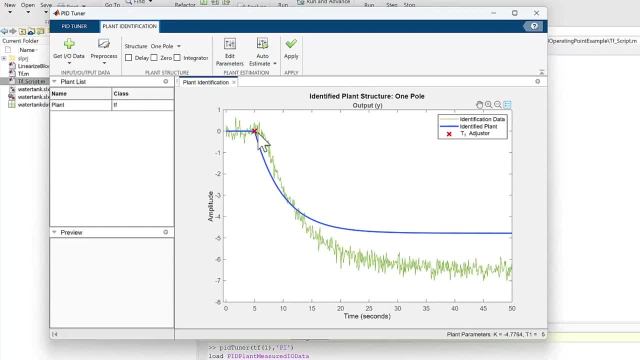 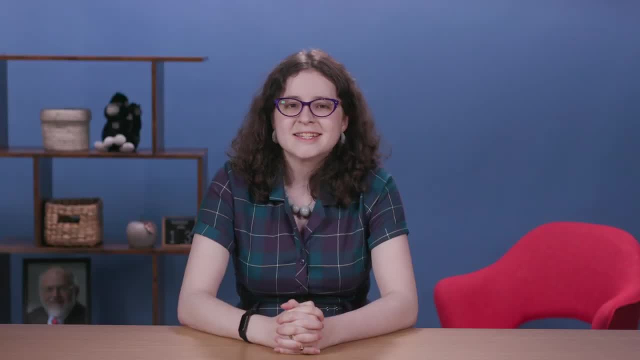 graphically. When we run the PID tuner, we can fit the model by site: Just click the curve and bring it to the response data. So that's the bird's eye view of LTIs, Obviously, as is the case of anything modeling related, 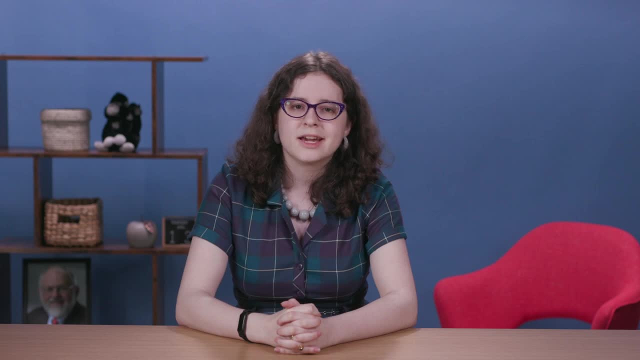 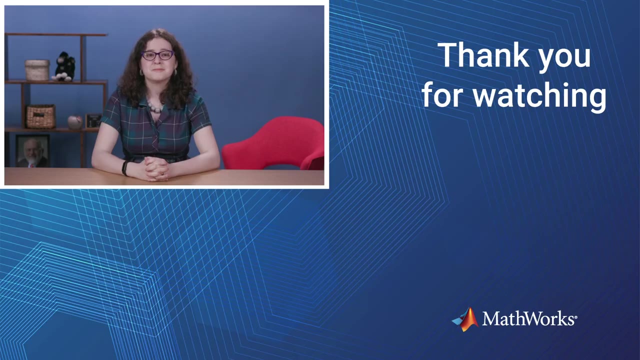 things can go horribly wrong When troubleshooting your system. I encourage you to check out the documentation on LTIs in Simulink and the documentation on the demos we did. For more information about controls design, please check out our series on understanding control systems.